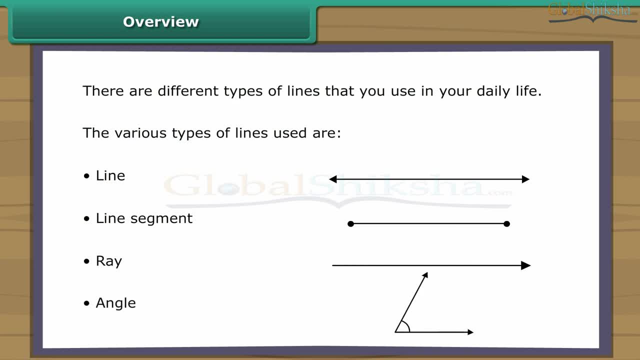 Angle. An angle is created with two rays having the same starting point. The starting point is called the vertex and the rays are called sides of the angle. Related angles: An angle is defined as the union of two rays that have the same end point. 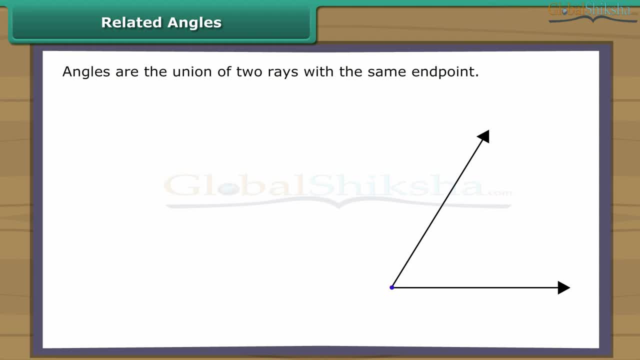 The sides of the angles are the two rays, while the vertex is the common end point. There are four types of angles. They are complementary angles, supplementary angles, adjacent angles and vertical angles. Now take a brief look on all the angles. Complementary angles are two angles whose measures add up to 90 degrees. 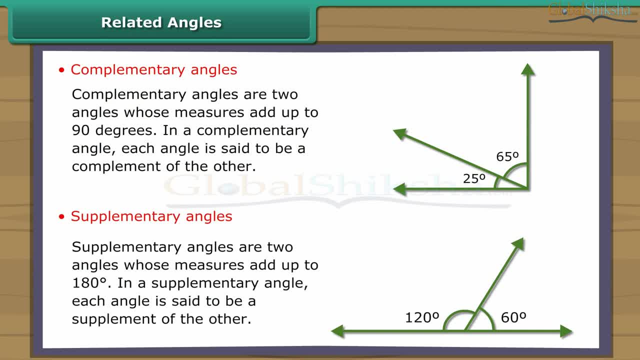 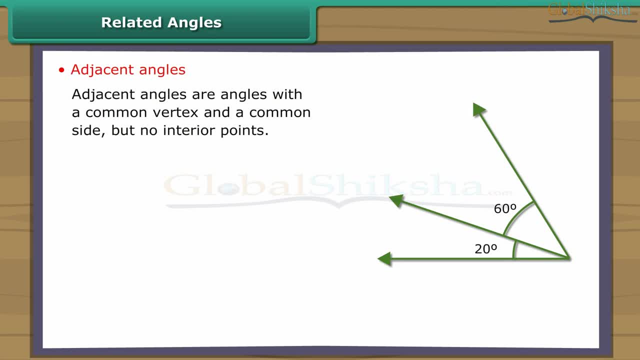 Supplementary angles are two angles whose measures add up to 180 degrees. Adjacent angles are angles with a common vertex and a common side, but no interior points. A pair of adjacent angles with rays as the non-vertex, The common sides, is called a linear pair. 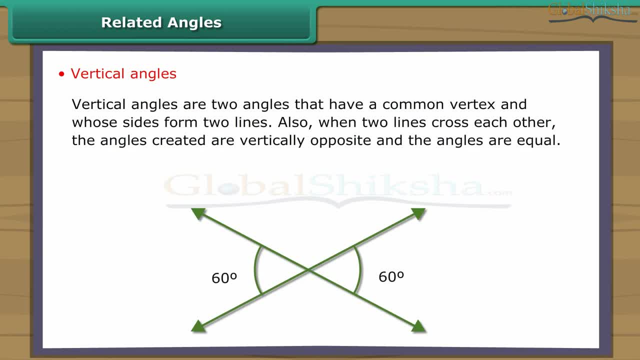 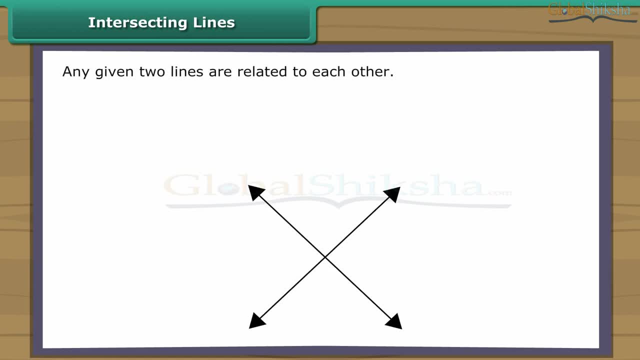 Vertical angles are two angles that have a common vertex and whose sides form two lines. Intersecting lines: Two lines are related to each other in different ways. Let us look at each way separately. Intersecting lines are lines that have one and only one point in common. 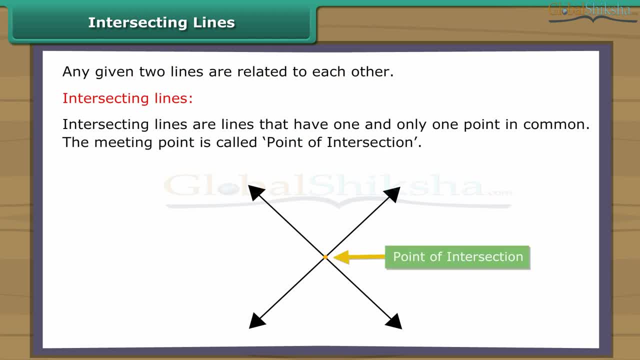 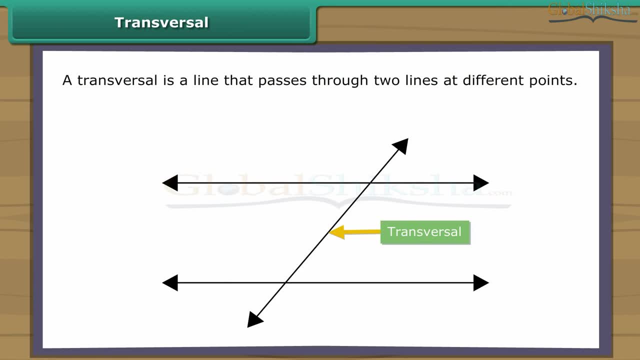 This meeting point is called point of intersection. Transversal. A transversal is a line that passes through two lines At different points. mostly a transversal produces several angles. Angles made by a transversal Transversals form seven types of angles. 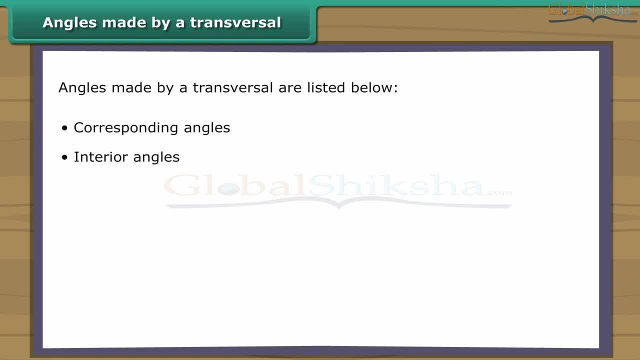 They are described as corresponding angles: interior angles- exterior angles. alternate interior angles- Constructive interior angles. alternate exterior angles- consecutive exterior angles. Click each button know more about above mentioned angles. transversal of parallel lines. when a transversal cuts through parallel lines, you will see that corresponding angles 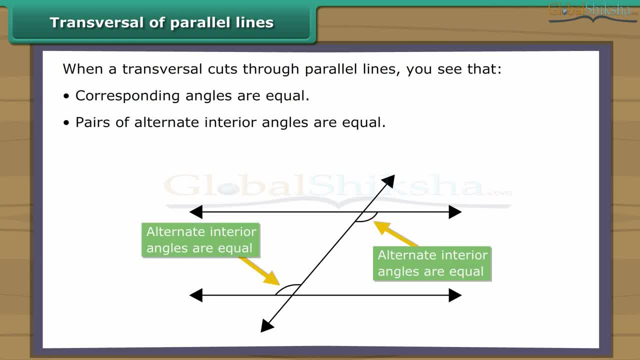 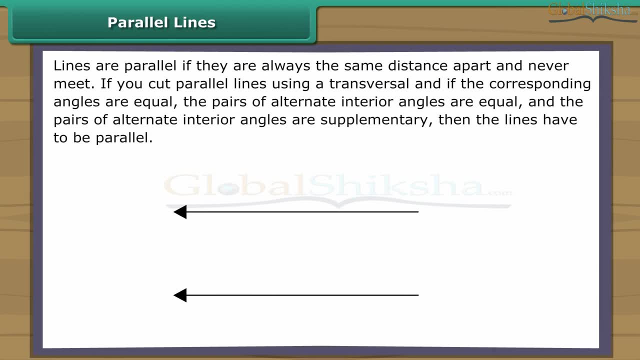 are equal. pairs of alternate interior angles are equal. pairs of interior angles are supplementary parallel lines. lines are parallel if they are always the same distance apart and never meet. you can also check if lines are parallel by cutting the lines using a transversal, if the corresponding angles are equal.